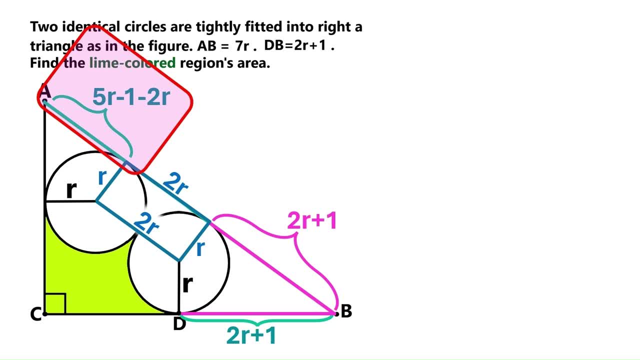 segment over here is 5r minus 1 minus 2r, Which equals 3r minus 1.. These two segments are tangents with a common point of origin, So they are equal. And this segment is also 3r minus 1.. Now let's. 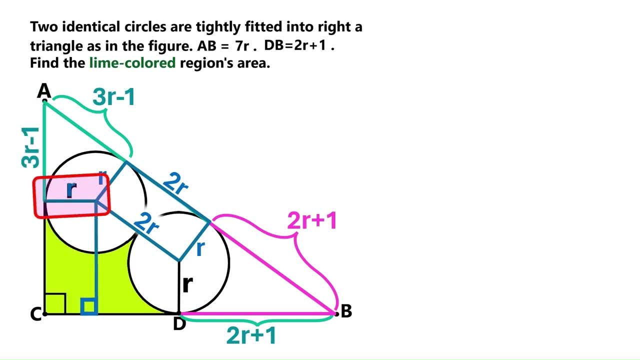 draw this line that's perpendicular to the triangle's base. Next, we'll take this r and project it to here. Let's draw another perpendicular line here. Now we'll take this r and project it to here. This shape is obviously a square, So this angle must be 90 degrees And its opposite angle must. 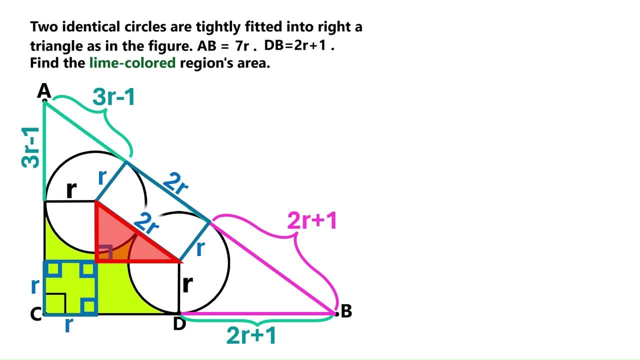 also be 90 degrees, And this little thing in the middle turns out to be a right triangle. Now let's name this angle alpha And we'll name this angle beta. We know that alpha plus beta is 90 degrees Because they are. 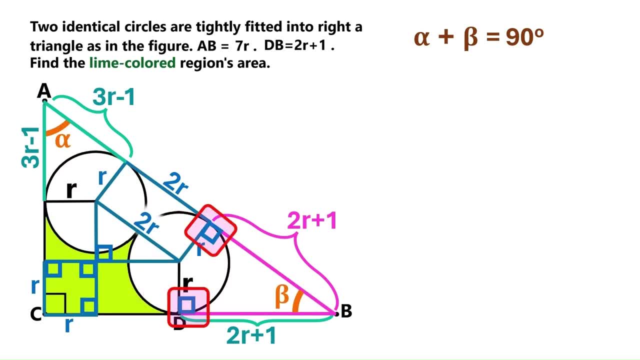 the angles of this big right triangle. Now these angles are both 90 degrees, And this shape's interior angles must add up to 360 degrees Because it has 4 sides, So this angle here has to be 180 minus beta. We've got two 90 degree angles here And all the angles around this. 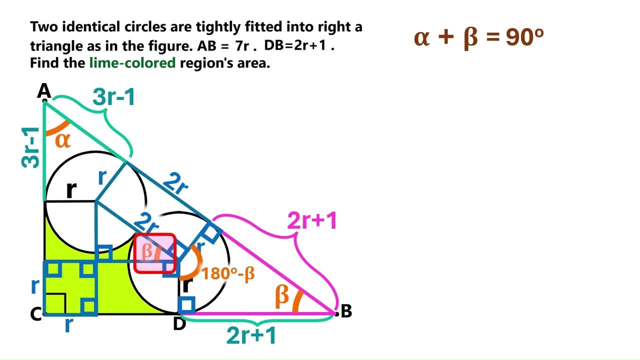 vertex must add up to 360 degrees. So we can conclude that this angle is beta And this angle has to be alpha, Because we know this is a right triangle, And alpha plus beta is 90 degrees. Now we'll call this side x, And this segment over here is also x, And we'll call this side y. 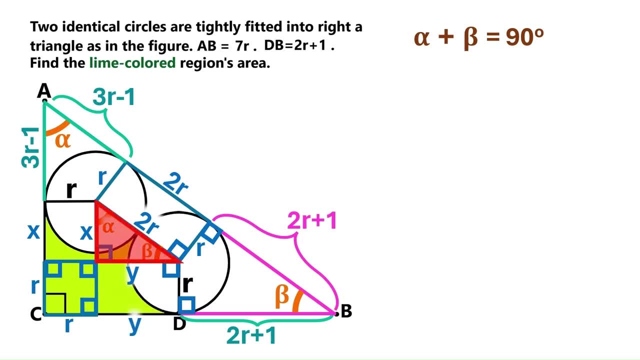 And this segment over here is also y. Now, this tiny right triangle is similar to this big right triangle Because they have the same angles. That means these two sides are proportional And we know this side is 7r, So let's put that value here. And its counterpart has a length of 2r. 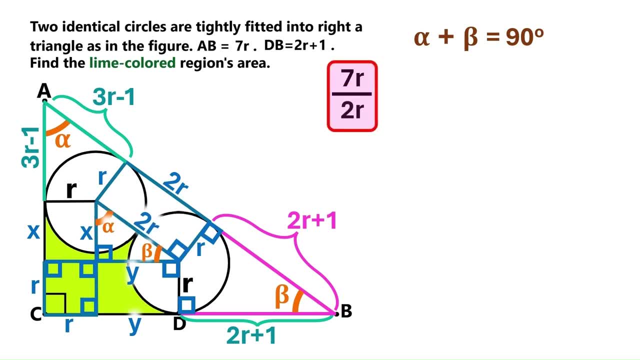 So let's combine them into a ratio Like this. Now this of course becomes 7 over 2.. These two sides must also have the same proportion. This side's total length is x plus 4r minus 1.. Let's put that over here And its 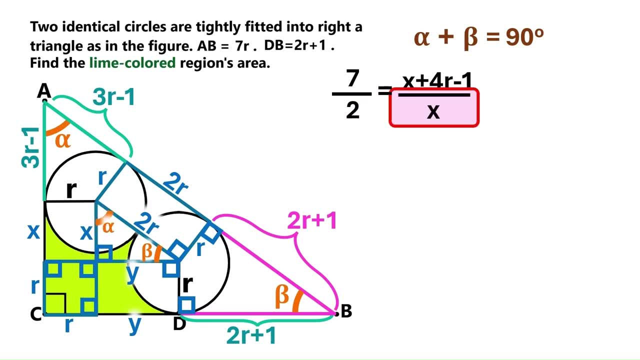 counterpart is simply x, So the denominator will be x. Now let's do the same for this side. The total length is y plus 3r plus 1.. And we put that over here And its counterpart is just y, And we'll. 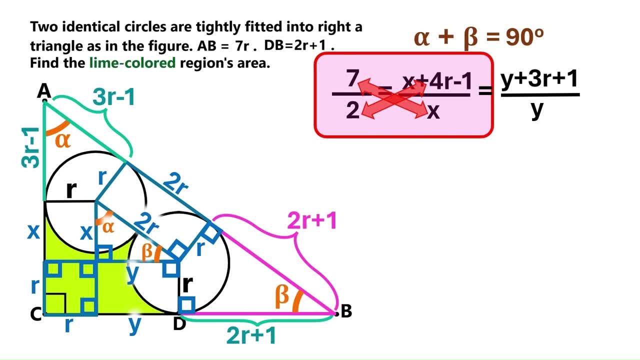 put that below the fraction line. Now we can cross, multiply this stuff over here. I'm doing the math for you And we find that x equals this. Let's put this finding up here and replace these x's with that. Next we cross multiply this stuff Again. I'm doing the math And it turns out y. 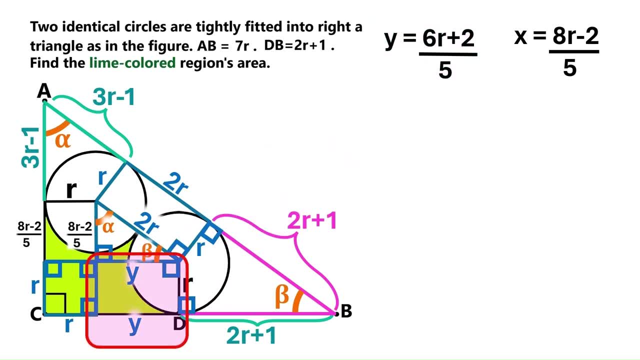 equals this. Let's also put this finding up here And replace these y's with what we found. Now we've got this right triangle And that means- Yes, you guessed right- Pythagorean theorem. It states that the sum of the squares of the shorter sides of a right triangle equals the square of. 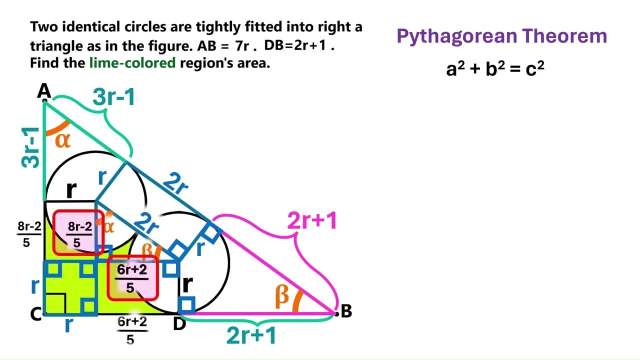 its long side. Now, these are the short sides in this right triangle, And these are the short sides in this right triangle, So let's take the squares of both. And this is the long side, So let's take its square as well. Next, we open up the brackets and we get this crazy equation: Let's add the. 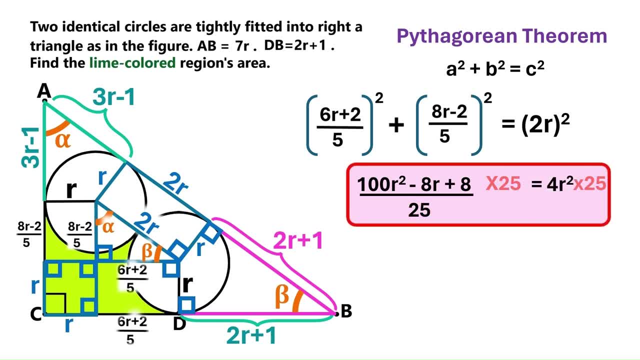 like terms together And it becomes this: We multiply both sides by 25. And things get neater. Let's get rid of the identical stuff on both sides And then take this 8 to the other side, Where it becomes minus 8.. We divide everything by minus 8.. It turns out r is 1.. Beautiful number. 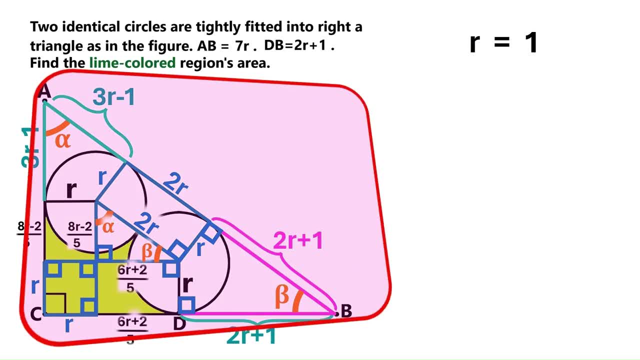 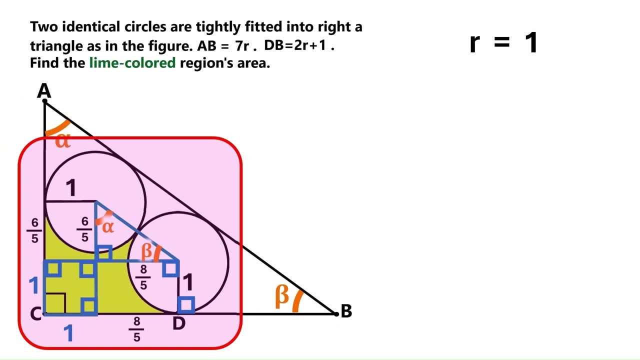 Let's keep this super important finding up here And let's replace all the r's with numerical values And let's delete the stuff we don't need anymore. Now I'll take this part and zoom in so that you can see everything clearly. This is the area we need to find, And to do that we must find. 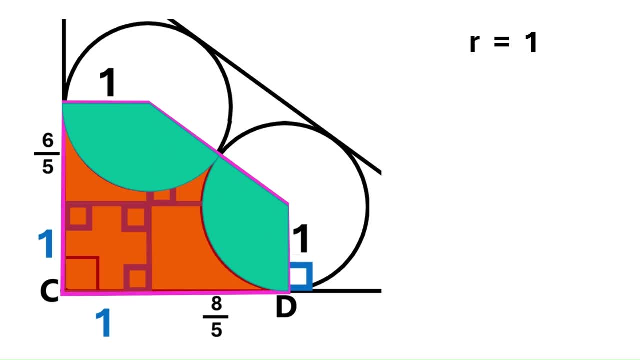 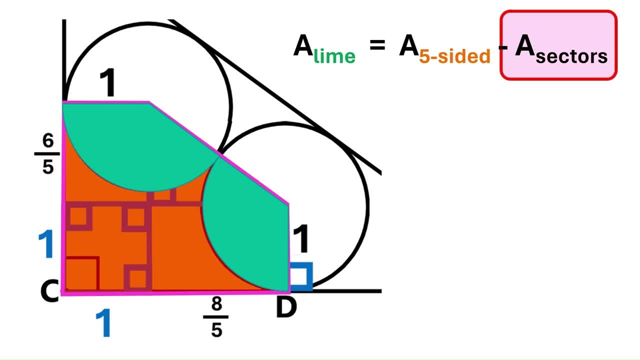 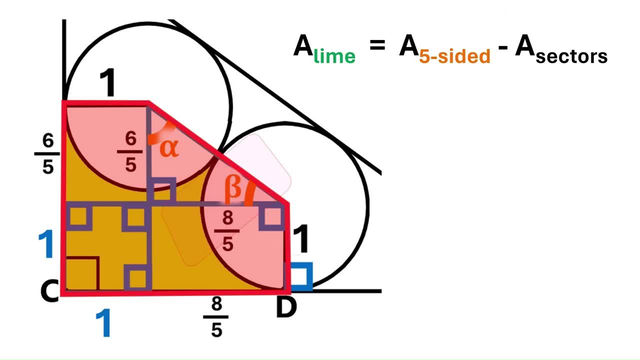 help with the calculations. Go ahead, son. Hi everyone, I'm gonna calculate some areas Now. we multiply one by one And the area of this square is 1.. We multiply. What is this, Son? we multiply them and divide it by 2 to get the area of the triangle, And it's 24 over 25.. Can you do the? 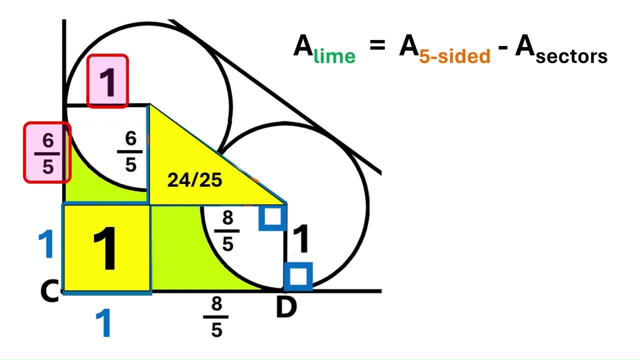 others. Yes, no problem, 6 over 5.. 5 over 5 is 1.. And we find the area of this rectangle And it's 6 over 5.. And 1 times 8 over 5 is 8 over 5.. 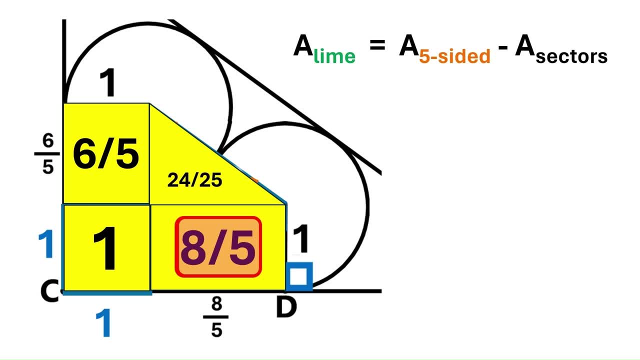 And that's the area of this rectangle, And you add them up, dad. Thank you very much, son. I'll carry on from this point. We add up everything we found And the total area of the 5 sided shape turns out to be 119 over 25.. We can now change the 5 sided area in this equation to that value. Next, we need: 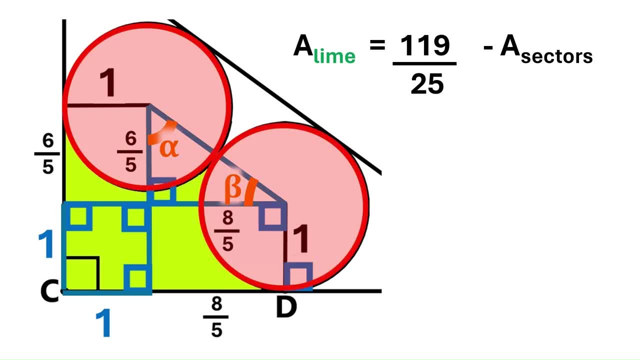 to find the area of these two circular sectors And they belong to identical circles, So we can basically put them together like they were sectors of the same circle. And they include these angles, alpha and beta, Which add up to 90 degrees, So we can simply replace them with a right angle. 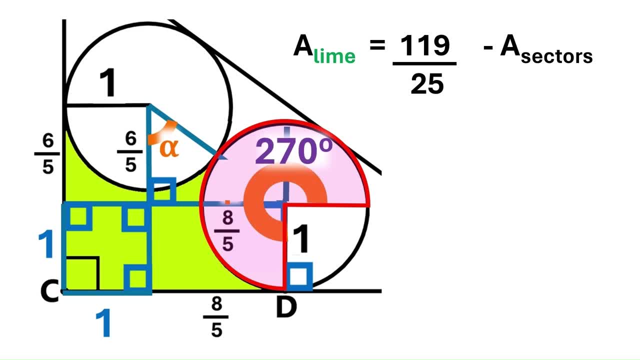 We get this big circular sector with a 270 degree angle. This is the formula we'll use to find its area. And we know r is 1.. So we can replace this r squared with 1.. We do the math And the total. 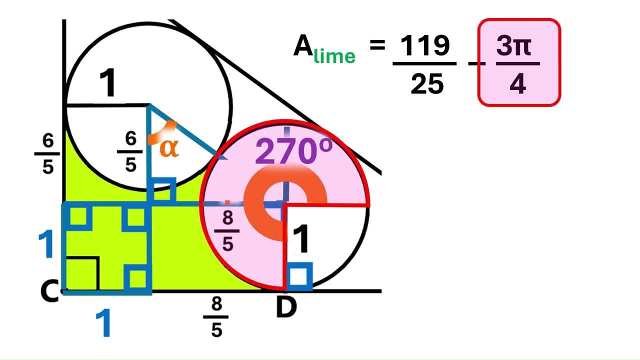 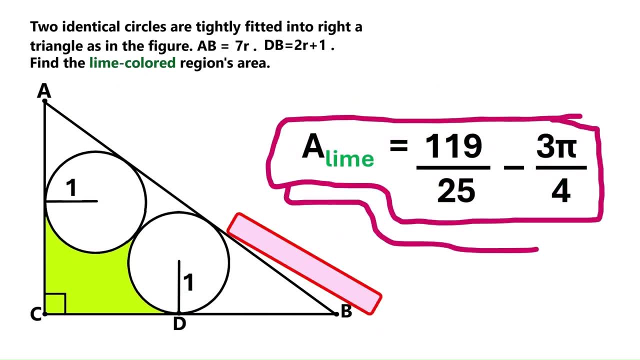 value of r squared is 1.. We replace this area of sectors with that value And there we are. We've found the area of the lime colored region. It's 119 over 25 minus 3 pi over 4.. So if you enjoyed, 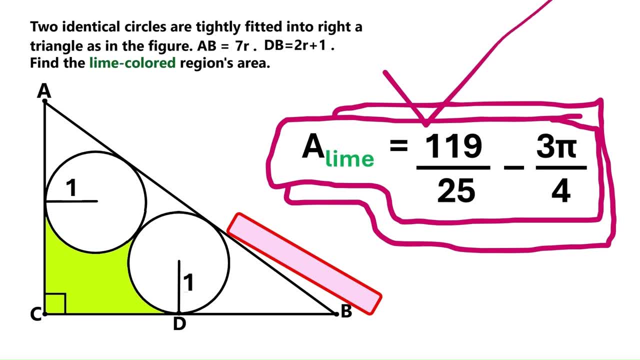 this video. please make sure you push the like button And don't forget to subscribe to our channel for our future videos. Have a good day And see you soon. 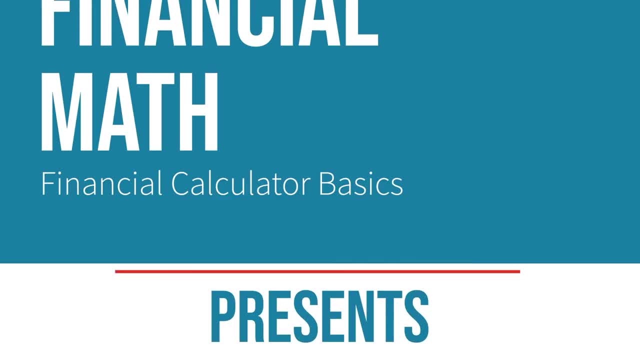 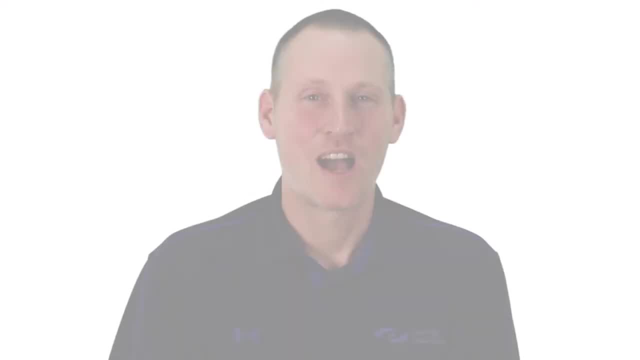 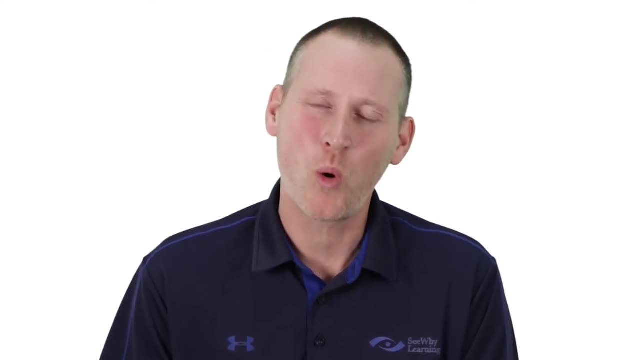 My name's Corey, one of the senior trainers here at CY Learning. Whether you're new to the industry or a seasoned veteran, it's important that you know how to do financial math. It can help with many industry courses and, more importantly, when working with clients. Now the best way to learn. 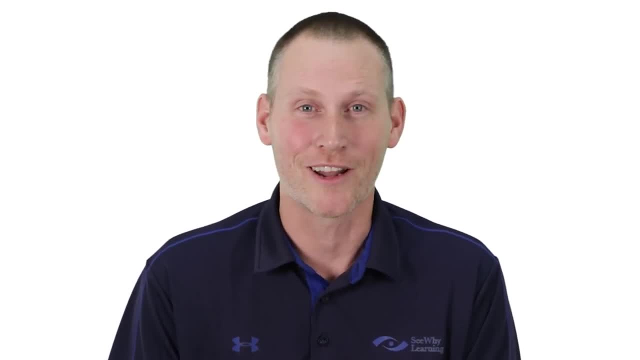 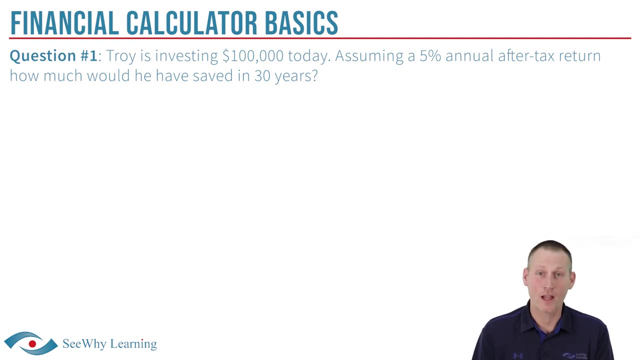 financial math is through practice, so let's roll up our sleeves and get started. Question number one: Troy is investing $100,000 today. Assuming a 5% annual after-tax return, how much would he have saved in 30 years? Well, there are a number of ways that this can be.